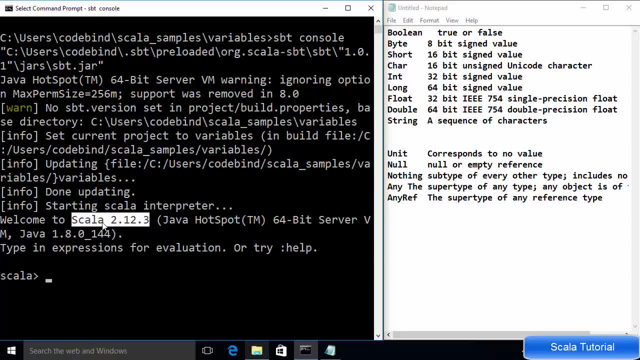 the version of Scala which it's using. So we are using Scala 2.12.3 right now. So let's talk about the data types which we can use in Scala. So these are some of the basic data types we can use in. 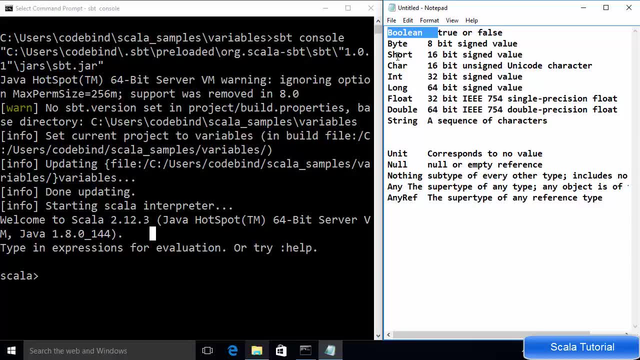 Scala, So we can use boolean, byte, short char, int, long float, double and string As data types. there are some more data types. which are these data types which are unit, null, nothing, any and any ref? These are some of the advanced data types and we will talk about them a little. 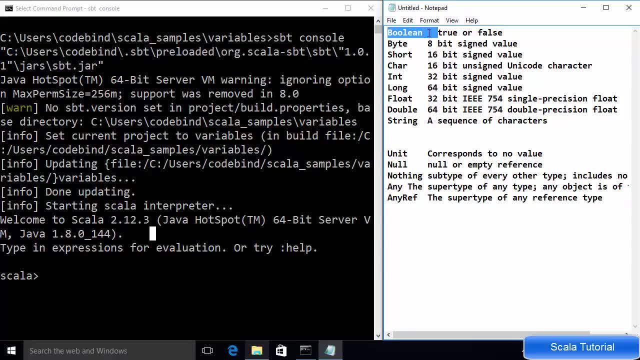 bit later So we can see here boolean. as you already know that it can be a true or false value. Byte is a 8 bit signed value. Short is a 16 bit signed value. Char is a 16 bit signed unicode character. Int is 32 bit signed value. Long is 64 bit signed value. And then you 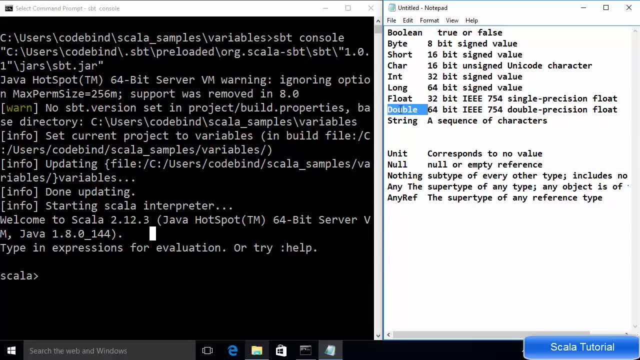 have for single precision float or double precision float And at last we have string, which is a sequence of characters. Now how we declare variables in Scala. So in Scala you can declare variables in two ways. So let's see the first way of declaring variables. 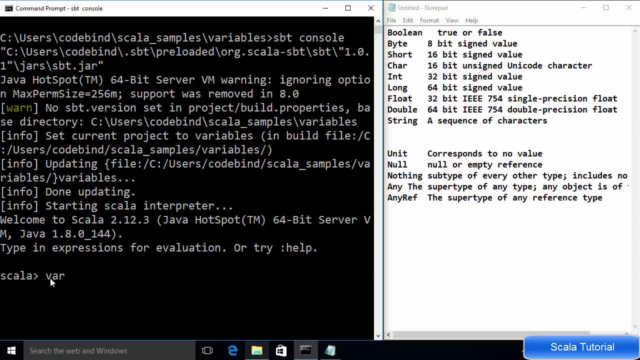 The first way of declaring variables is using var And var. whenever you use var, that means it's a mutable value. That means you can change the value of this variable later. Okay, so mutable variable means you can change the value of this variable later. So you write var. This is a keyword Then. 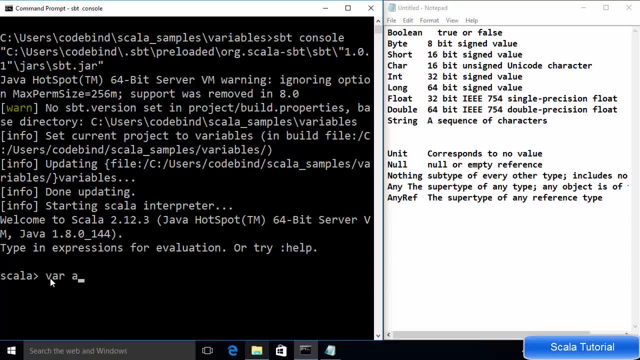 you give a name to your variable. For example, I use a simple name A- And then you give the data type after this colon. So then you use colon and the data type- For example, I use int as data type- And then you initialize your value with equals and then 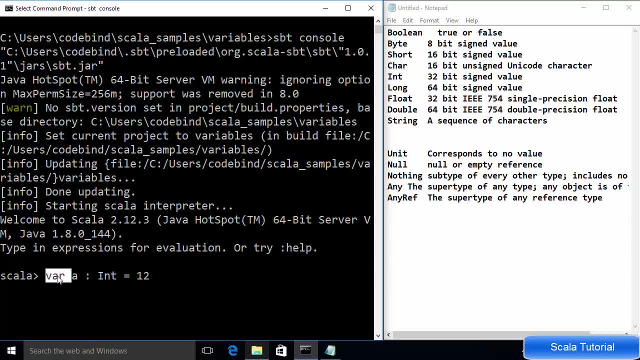 whatever number you want to give here. So you use var, a special keyword which indicates that this is a mutable value, Then a variable name, Then a colon, Then a data type, And equals the value of data type. Right Now you can use the semicolon to end your line of code, or 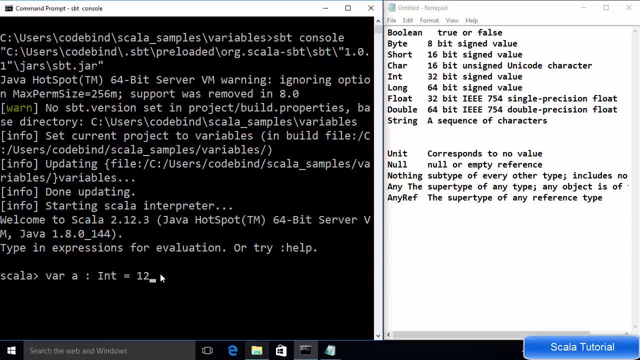 you can leave it without a semicolon, It doesn't matter, Right? So when I just press enter and it says a colon, int is equal to 12.. So this basically means that we have declared a variable called a, whose data type is int. 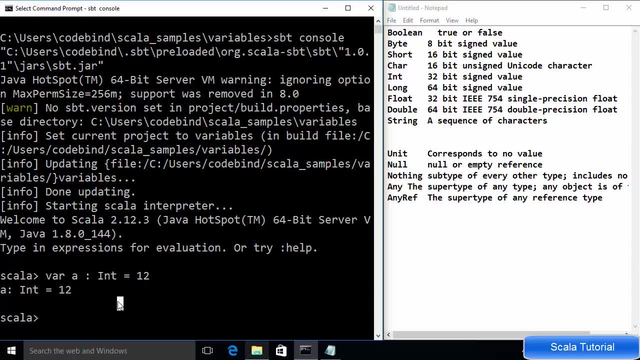 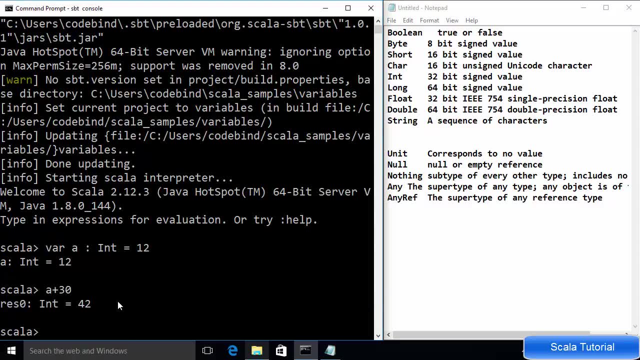 We have assigned the value of 12 to this variable. a Right. Now you can do a plus 30, for example, and then press enter, and then you will get the value for this. So 12 plus 30 is 42, and you will see. 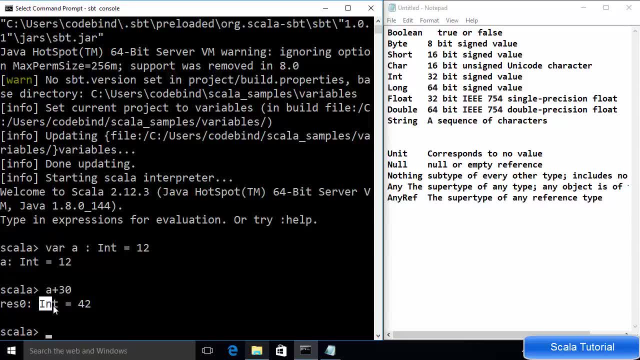 the result and the result of data type you can see here. And if you are wondering, what is this, This is a temporary variable in which your result will be stored And then, at last, this is the sequence which will increase one by one. So result: zero. This is a temporary data. 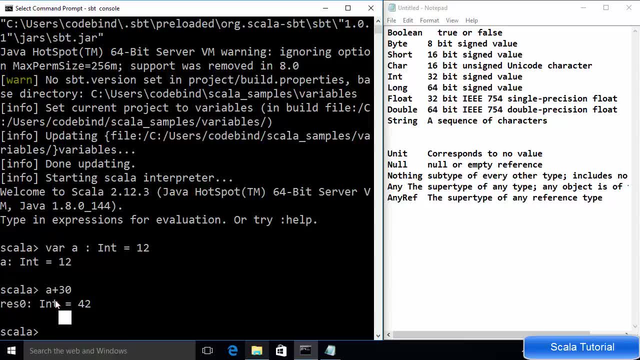 type and it will start with RDS- for example zero- And when you will evaluate more expressions using this scholar rappel, then you will see this number will increase by one every time you do this. So, for example, when I do a plus 40 now, then you will see RDS one. That means this value, at last, is increased. 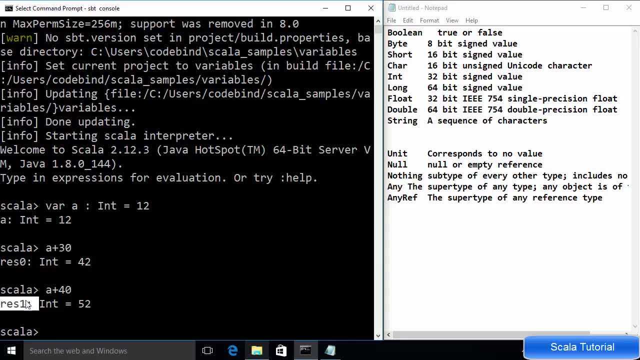 and this is a temporary result variable which is created by scholar for you. So you can declare a variable like where, or mutable variable, and then you can declare a variable as an immutable variable. So for those immutable values we use a keyword called well and then your variable name for. 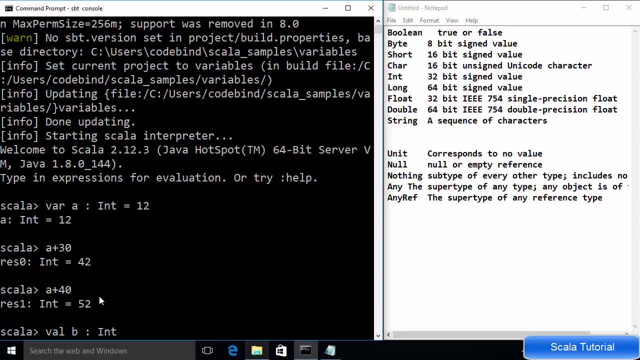 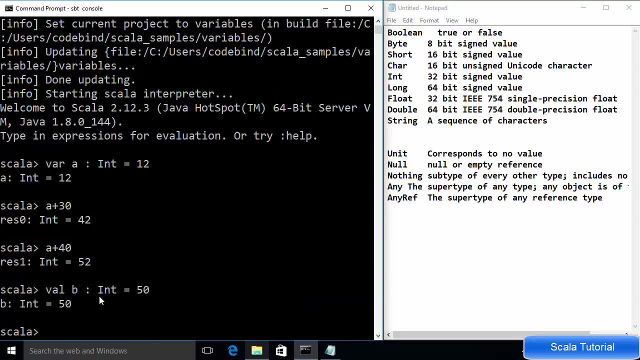 example B colon, and then your data type, for example int, and then you initialize your variable, for example 50. Okay, And then press enter and you can see this variable is declared. is that when you declare a variable using well keyword, then its value cannot be changed. So this means that value of variable B is constant. 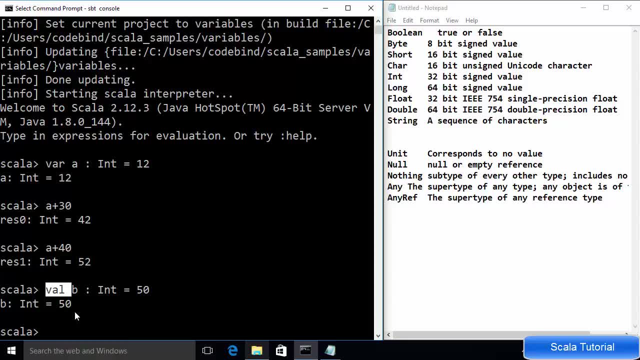 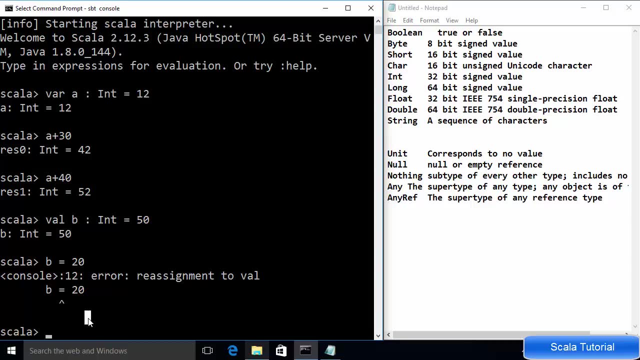 and it cannot be changed, or it's immutable. That means it cannot be changed. So, for example, I use B is equal to 20. now It will give me the error and it says reassignment to well. On the other hand, when I do, A is equal to. 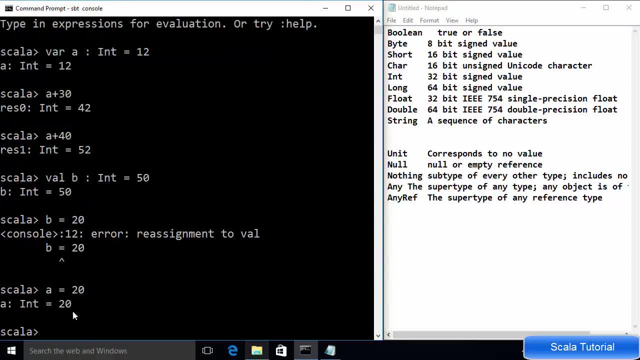 20 and then press enter. it's totally fine, because we have used a keyword called var before it. That means the variable value can be changed, Right? So when you use var, the variable value can be changed. when you use well, the variable value cannot be changed. And now let's see in the folder: 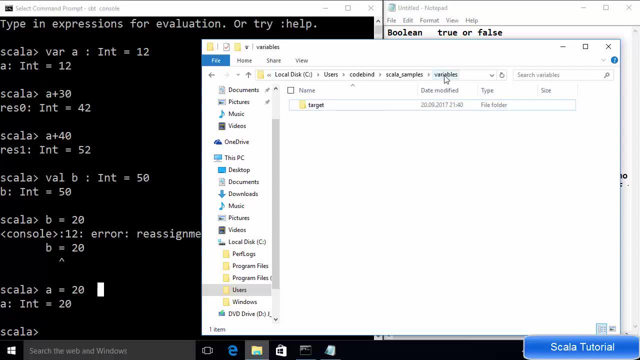 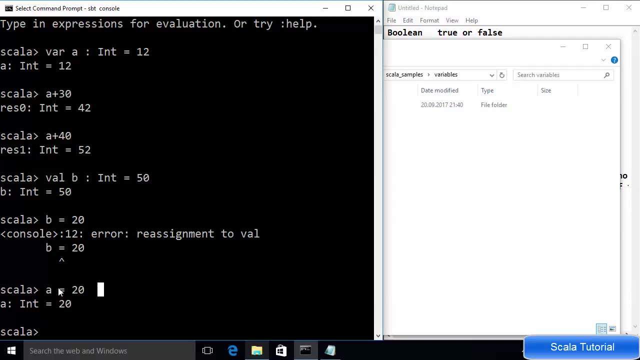 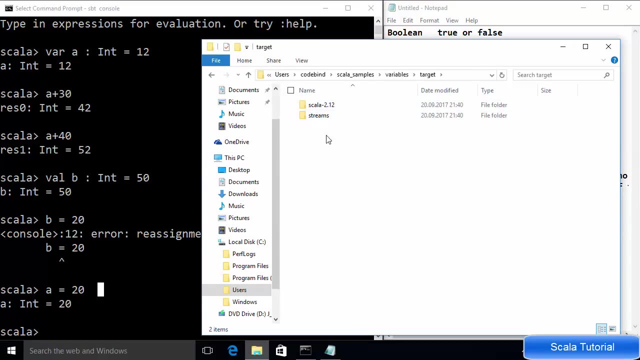 in which we are working in. So you can see we are working in the variable folder and earlier it was empty. But when we, you know, start our rappel in this folder, there is a folder called target, created automatically in this folder And here all your, for example, intermediate files will be created for. 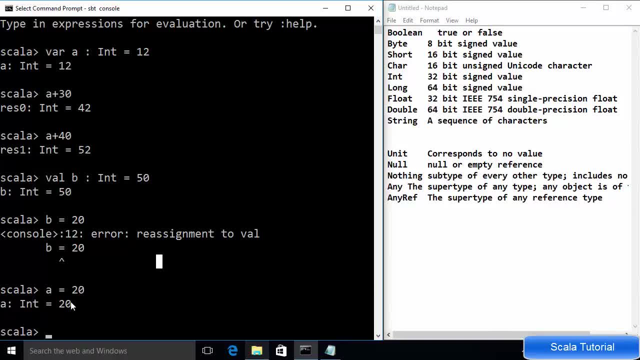 Scala and they will be compiled and they will show the result here on the Terminal. So always keep in mind: Scala is not interpreted, It's a compiled language. Now let's say you declare a variables- var C, colon int, for example- and we are not initializing this value. 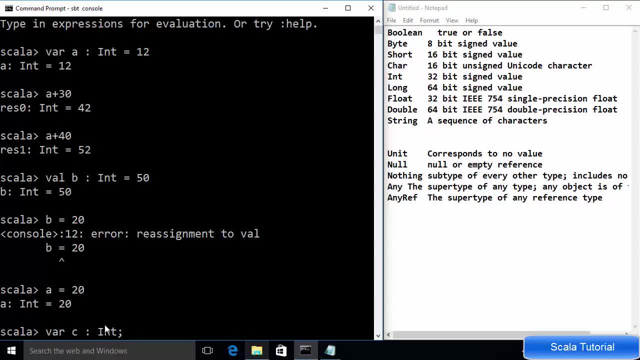 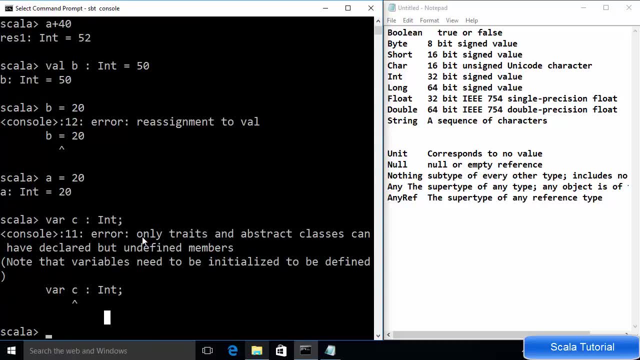 OK, So we haven't assigned any value to C, and then we press enter and it says error. That means you need to initialize these value whenever you are using this rappel. Now there is a special feature about Scala, and that is data type recognition by its initialization value. OK, 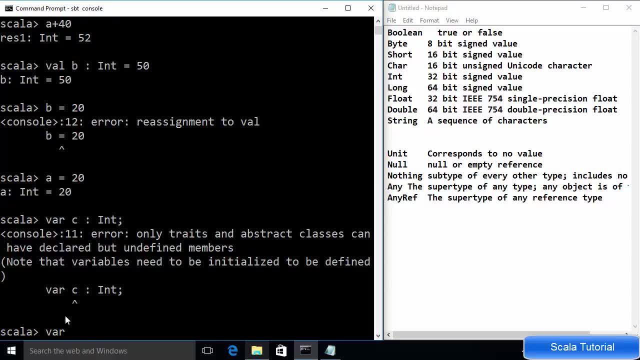 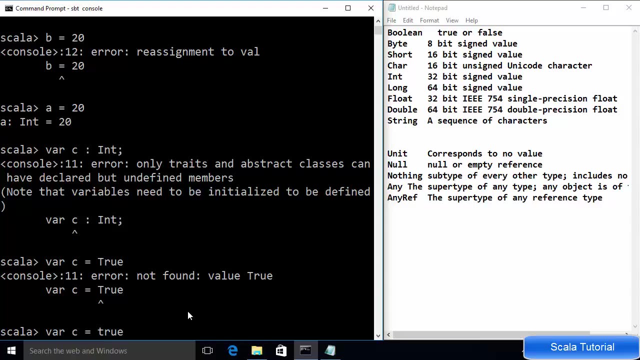 So, for example, I declare a variable C once again and then I don't give any data type to it. I will just say: is equal to true. Let me correct this, It should be true with smaller t, OK, And then press enter and then you will see that Scala recognizes the data type by the. 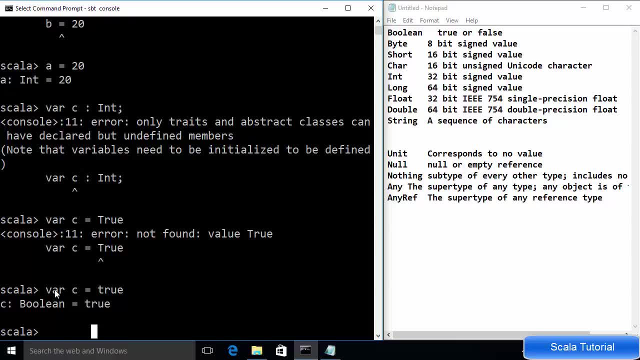 initialization value: OK. So for example, you initialize, the value is equal to true, That means Scala interprets that it's a Boolean data type. so we can see here: Boolean data type is assigned to C. here Now, for example, I can declare: var D is equal to some number. So for example, let's say: 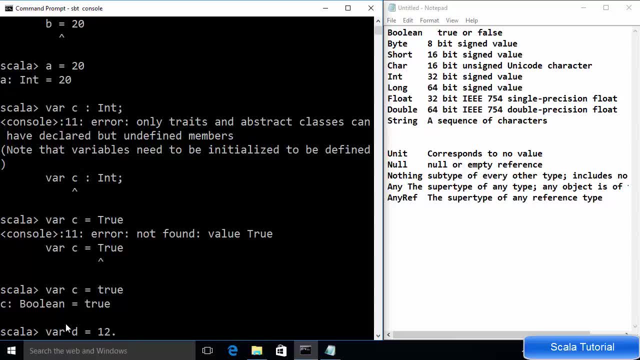 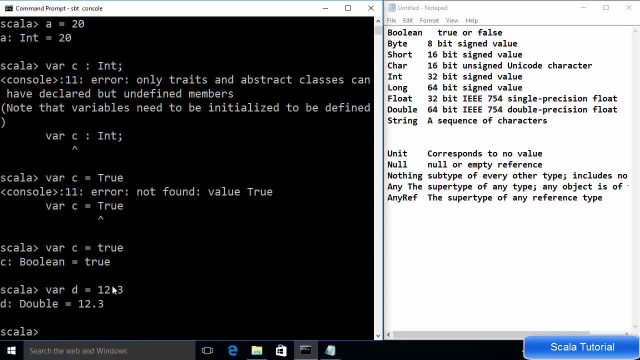 I define a number called twelve, point three. This is a float value and we say Enter. So by default it recognizes this decimal value as a double data type. Right, It doesn't recognize this by default, this decimal number, as a float value. So if you want to define the variable, 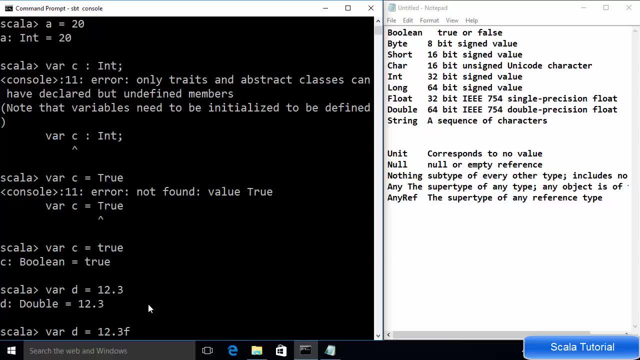 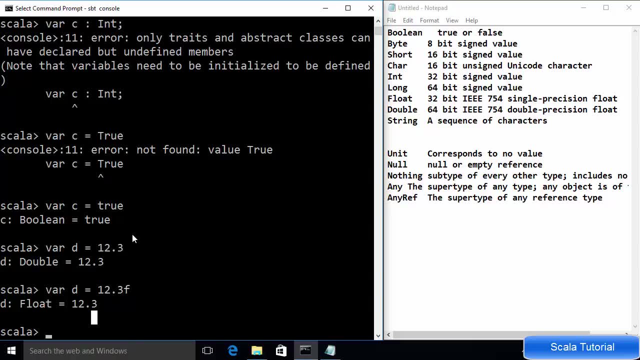 as a float value. you can just write F here and now it will recognize this value as a float. OK, So what this indicates? that Scala interprets its variable data type from the initialization value, whatever we assign as an initial value to a variable. So if we assign true, the data type, 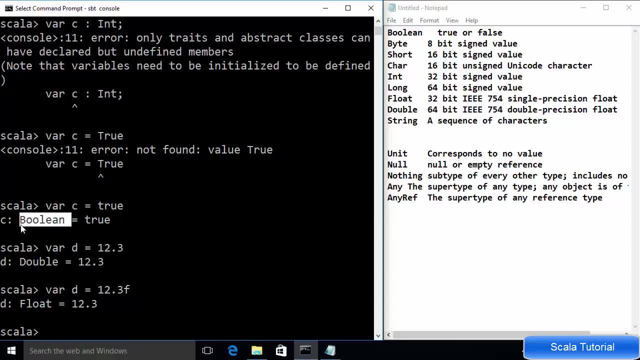 will be automatically inferred as Boolean Right. If we assign any integer, then data type will be automatically assigned as an int. If we use a decimal value, the default data type is double, but we can also declare a float data type with these kind of initial values. 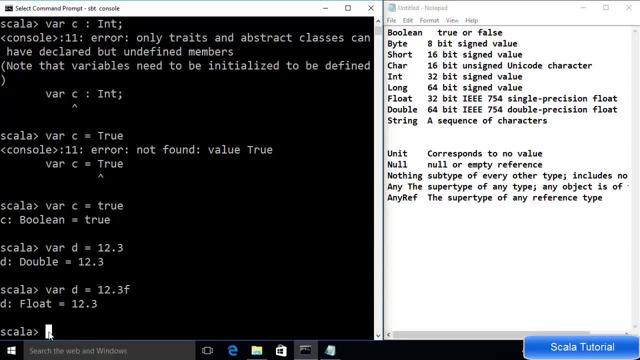 Now in Scala you can use multiple expression using a curly bracket. So for example, I declare immutable variable X and then I use these curly brackets and inside those curly bracket I can declare some variable. for example val, A colon int is equal to 200, and then I can separate those. 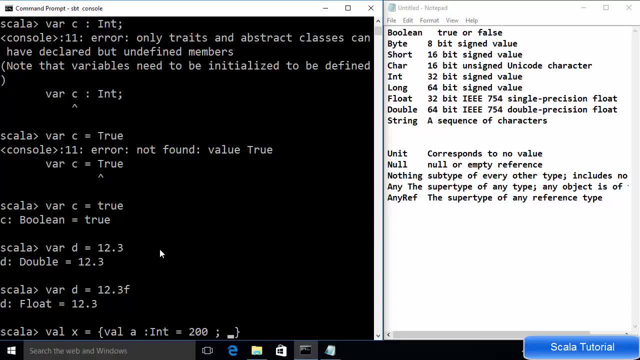 expression by semi colon. so I can declare a second variable. for example, val B is equal to 300 and semi colon, and then we can just return the result using the last expression. So for example, you want A plus B here, so we can just write A plus B and then press enter and you 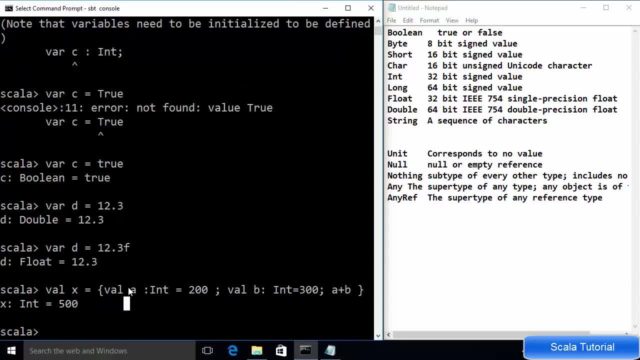 will get 500 and what this means. this means that we have declared two variables. variable A is equal to 200, variable B is equal to 300. both are integers and the last expression returns the result. Okay, So this will add those two values and assign the value to the variable X. 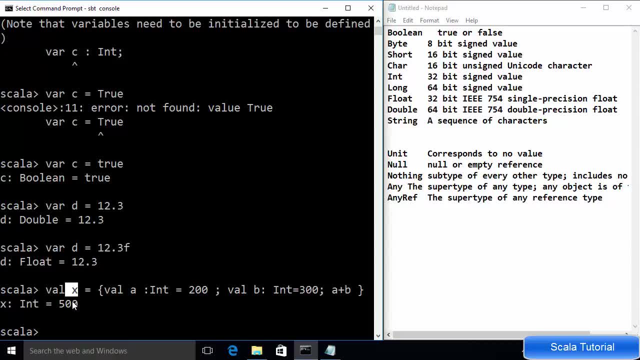 Okay, So the final value of X will be 500.. Okay, So the last expression is the result which will be returned and assigned to the variable, and it's not necessary that you can declare only two variables here. You can declare any number of variables. 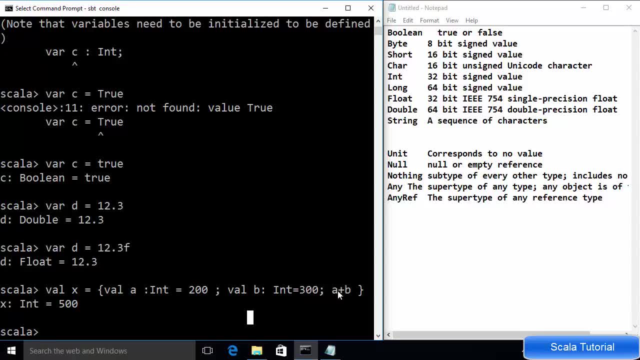 Here, but the last expression will evaluate the result and assign it to this variable. Okay, So, for example, if there will be ABC variable and if you want to do the addition of all three variables, then you can do that also. Now I said that you can separate these expression by semi colon, so this is one statement. 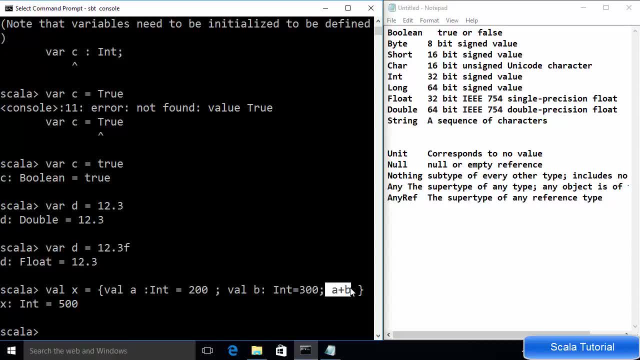 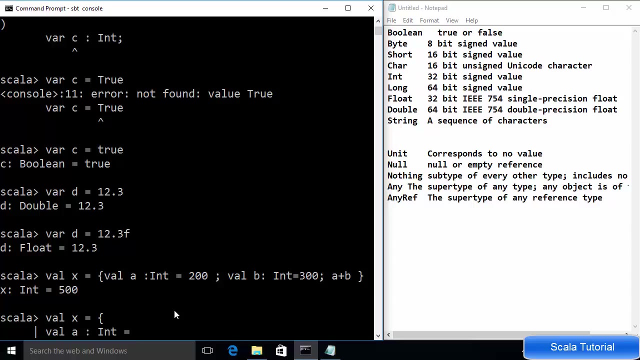 This is second statement, This is third statement. Right, So you can either use Semi colon or a next line. So, for example, same thing I want to do, so I will do. well, X is equal to, then curly bracket and then press enter, and then I can declare a first variable, for example: well, A is equal to 500 this time, and then press enter. 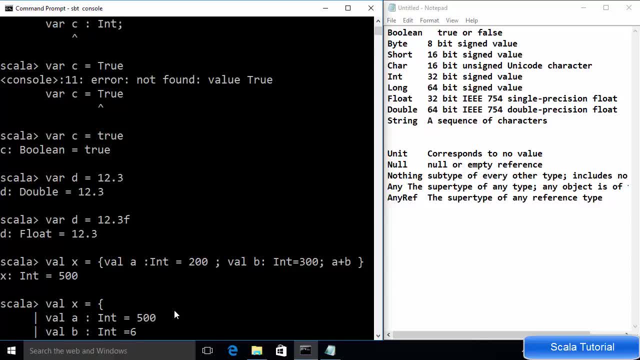 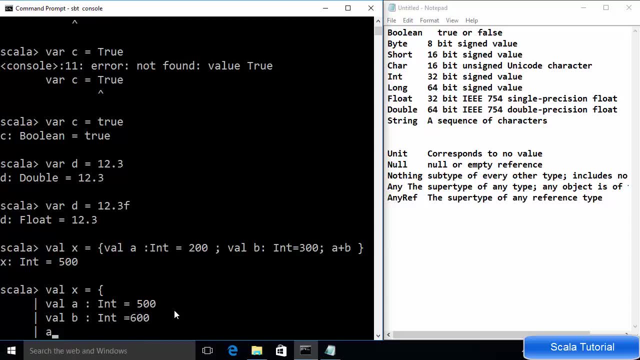 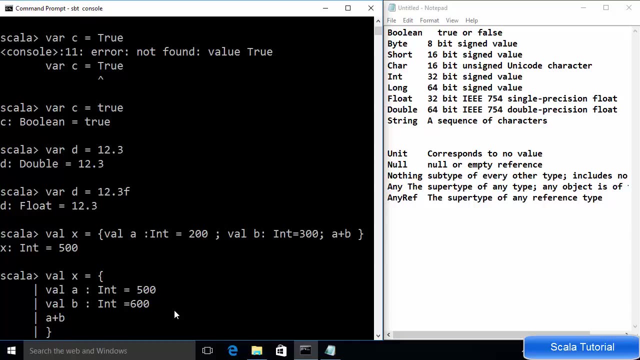 well, B is equal to 600 this time. and then press enter And then We will evaluate these two values, for example A plus B, and then press enter and then give the ending curly bracket, And once you press enter now, then you will see the result, and result is eleven hundred. 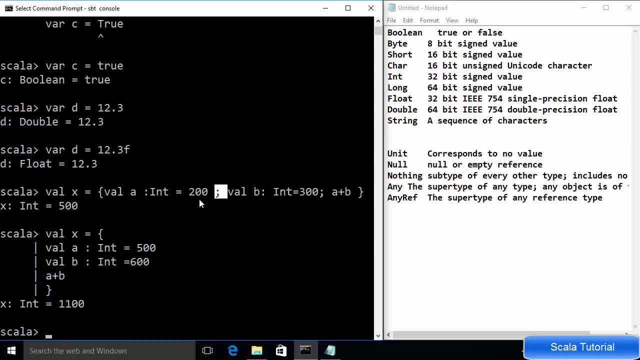 That means you can use semi colon as a delimiter or a new line as a delimiter. Now the last thing I want to talk about in this video is the lazy loading, or on demand loading. So generally you declare a variable Like this: so well, X is equal to 500. and then press enter and it declares a variable and it allocates the memory for this value and everything is good. 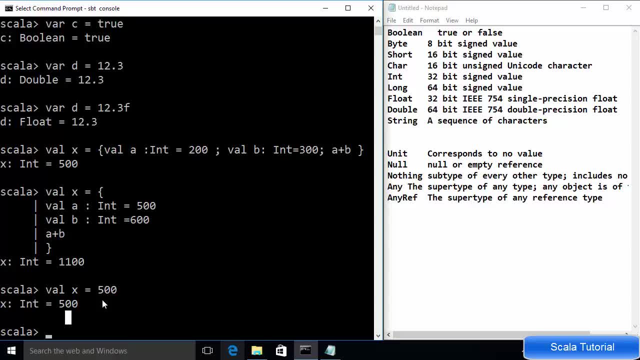 And now, for example, I want to do some arithmetic operation on this. So, for example, I do X multiplied by 30, right, and then press enter and it will give us the result. OK, Now let's say we Declare here a list, For example, list which contains millions and millions of values, right,